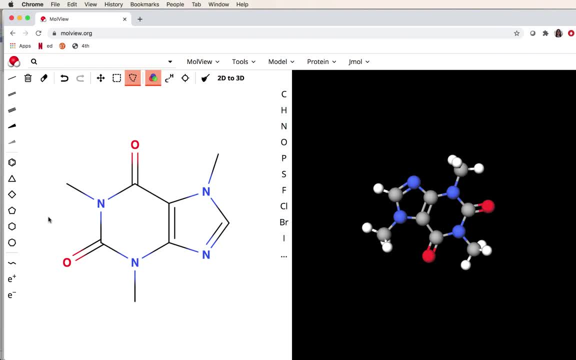 and this is a little bit of a problem with MoleView- is that the orientation of the molecule on the left isn't always the same as on the right. You'll notice that the big six-pipe molecule at the bottom is the first one and the second one is the first one. 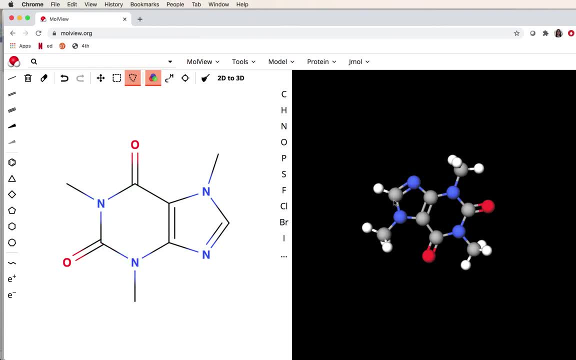 membered ring is on the left side of the molecule and here we have the five membered ring on the left side. So I'm going to go ahead and switch this around so that we can see what we're looking at here and it makes a little bit more sense. I'm going to flip it like this, just with our mouse. 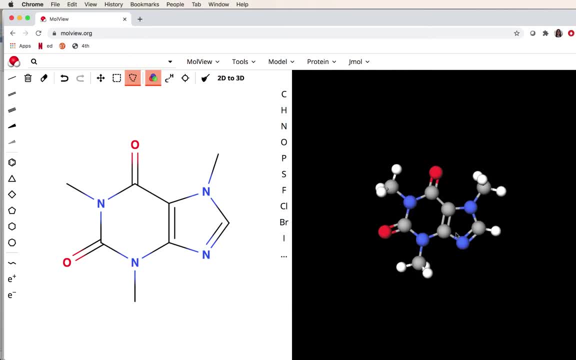 You're going to just click and hold with the mouse, and now that's a little bit better. Now you can compare the two structures. I'm going to use two fingers on the mouse to kind of zoom us up a little bit so it's more of the same size, and then that's a really useful thing to have to have the 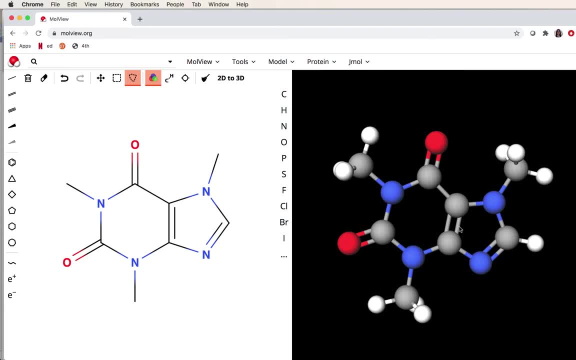 drawing on the left side and then the 3D structure on the right side. So let's get started and build our own structure in MoldView and then we're going to render it in 3D, which is the whole purpose of why we're adding this to the program To erase the caffeine, because we may not always want to look at. 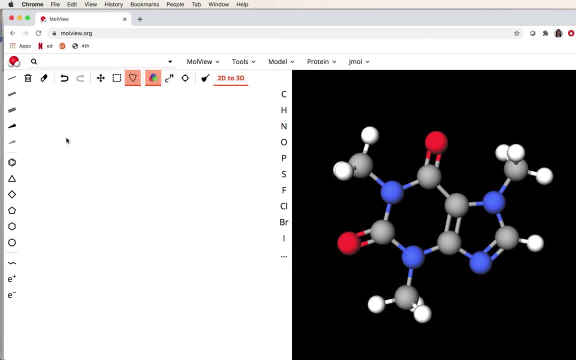 caffeine go over to the little garbage can here? just click it. That clears our screen and we're ready to draw a new structure On the left side. here you're going to see all different kinds of bonds. You can build a single bond. 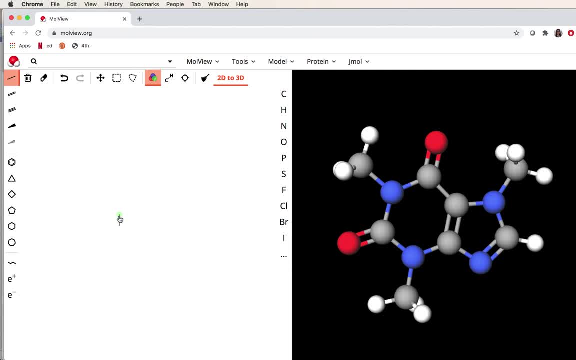 let's build a single bond, maybe just up and down a couple single bonds like this. I'm just clicking and holding, looking where the little green highlighted pieces. that's going to help us see where we are making our drawing. There's our double bond. let's add a double bond right here. Let's put a. 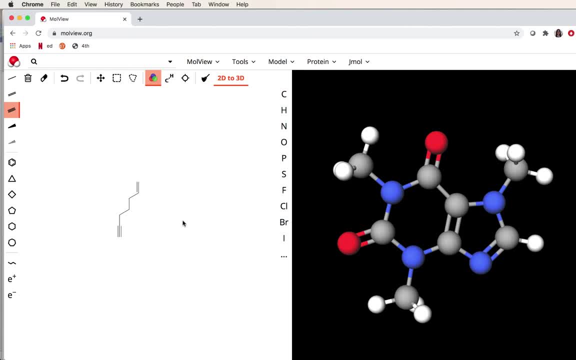 triple bond, maybe over here. So that's how we add the bonds. If we're interested in the stereochemistry, we can use these wedges. When we get to the stereochemistry chapters you'll understand what those are. but those are basically just single bonds. but they have to do with 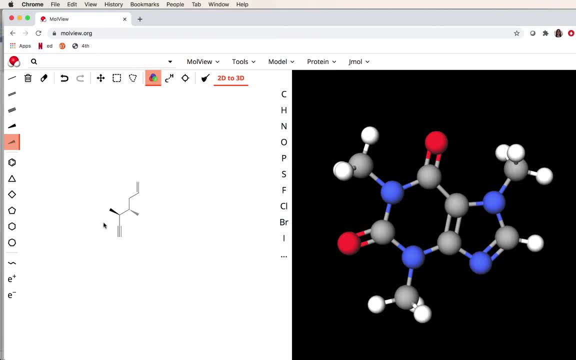 whether the bond is coming towards us or away from us. The solid wedge means it's coming towards us and the dotted wedge means it's away. I'm going to use my mouse to zoom up a little bit. We can also hit this button to zoom closer. That's another way of zooming in, so we can see what we're doing here. 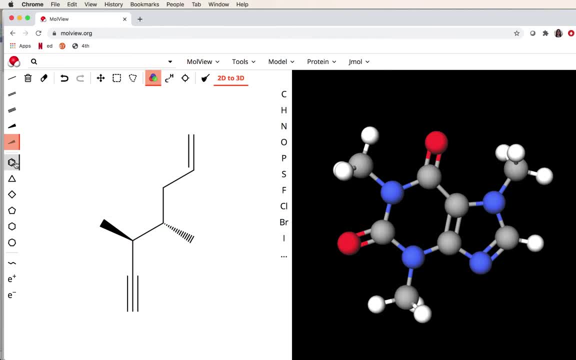 So now you can see our double bond, triple bond, our stereochemistry. Let's go ahead and add a little benzene ring to this thing. Let's maybe put a little benzene ring right here. So it's kind of, I think. 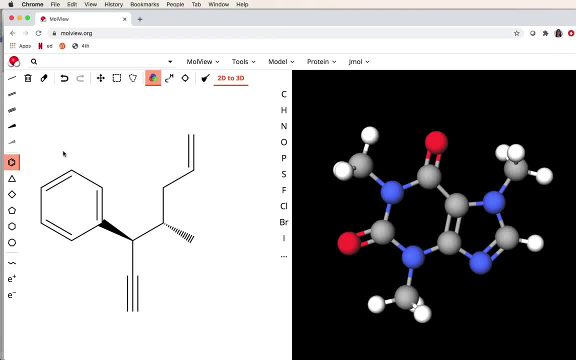 it's pretty intuitive how this works and, like I said, this is a free version of what are typically much more expensive molecular drawing software. So the one that I use to create the drawings for biochemistry literacy is called ChemDraw and it's extremely expensive. It's prohibitively expensive for my users. 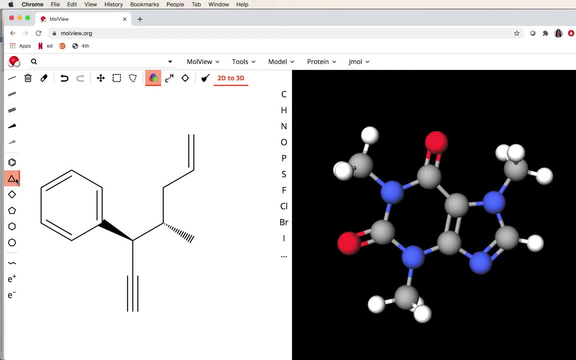 to be using, but this is a free alternative and it does have a few little kinks here and there, but for the most part it's going to be really great for you guys to use, Alright, so I'm just kind of making a creative structure. I'm just kind of adding some things on here and we can also add different kinds. 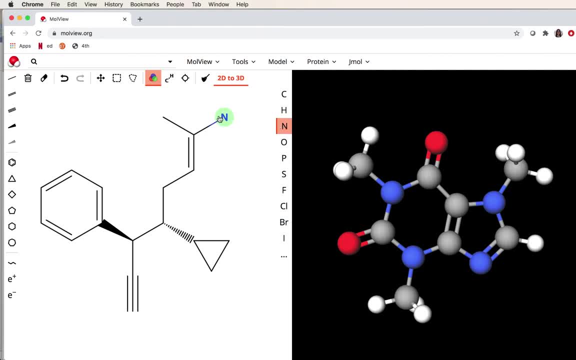 of atoms. So maybe we want an amine over here We can put our nitrogen and then we need some hydrogens, right? So what I'm going to do here is I'm going to click single bond and I'm going to click H, and now, whenever I add a single bond, 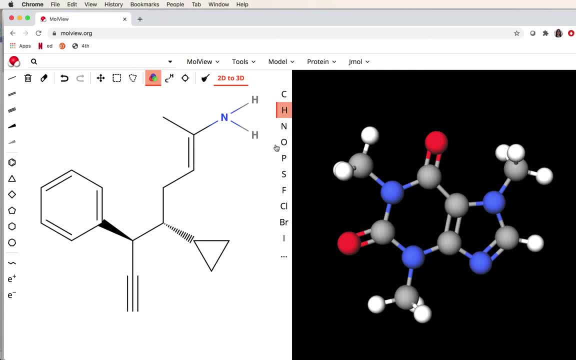 there's going to be a little H at the end. Hmm, that's nice, Let's go ahead and do the same thing with an oxygen. Let's add this, and we're going to add an oxygen at the end, and then we're going to go back and click the H. 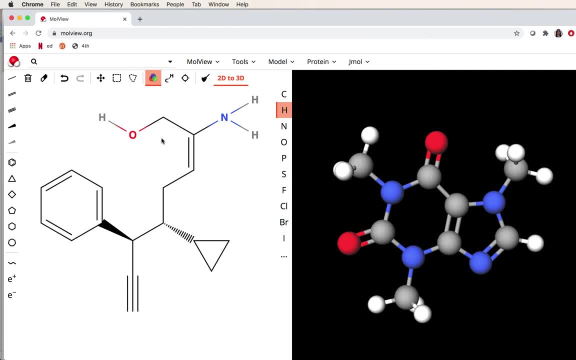 That adds an H to the end. So now we have a little alcohol, a little OH group there. So that's how you basically how you add atoms to this If we click this. I'm not going to do it right now. 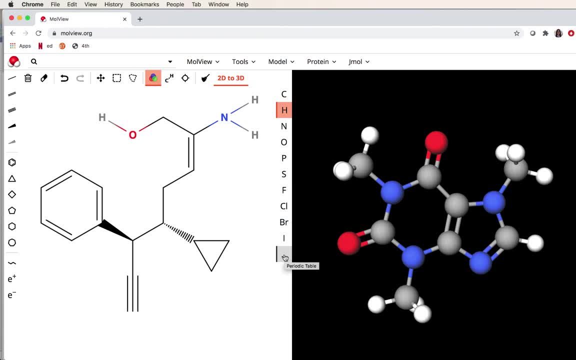 but if you click this you get the whole periodic table and you can put any atom you want. Not super useful for us for this program, because most of the atoms we use are already right here. We don't typically need, you know, uranium or something, So don't worry, worry about that too much. 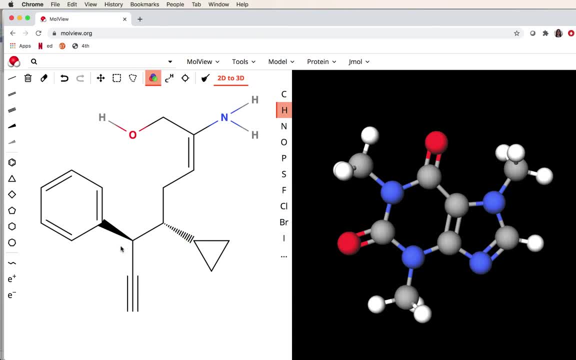 But that's the basic idea of drawing. There's a couple other things to know about. We can also add charges. So if we're interested in drawing amino acids, let's kind of we'll start over, actually before we start over. 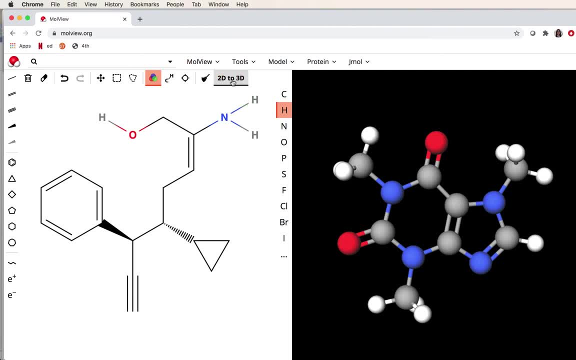 let's go ahead and render this in 3D, just to have a variety of things here. Once you've made this drawing- and it's great to draw, it's great to practice drawing, learn how to professionally draw things- we're going to go ahead and click 2D to 3D and that's going to get rid of our caffeine and it's going to give us. 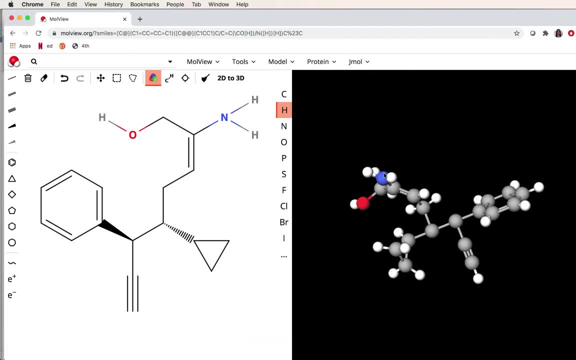 this gives us these error messages. I'm not really sure why, but it's going to give us a 3D version- and usually fairly accurate version- of the molecule that we just drew. So look how 3D this is. it's really cool. 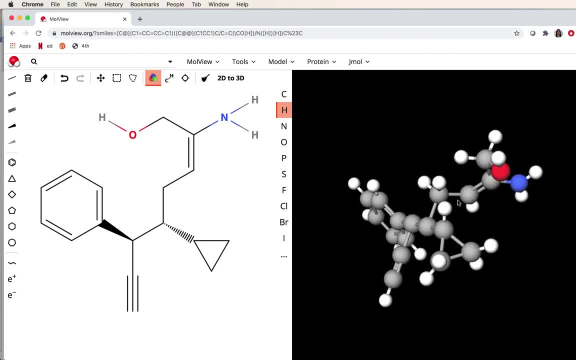 We see that benzene ring, And again the orientation isn't right, so I'm going to flip it over. It says little bit better. We can see that we have our benzene ring, our ring, over here. That's the benzene ring, same thing. And then we also have our little cyclopropane ring, which is this triangle. 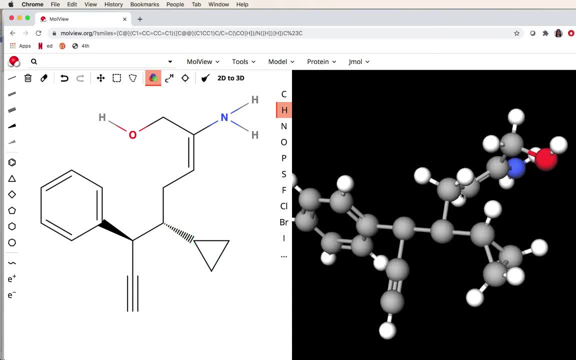 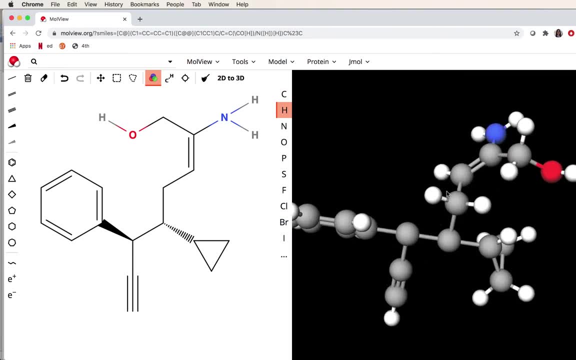 here That's the same triangle as over there. We have our triple bond, our double bond. you know all the different things we put in there. we can see in our cool 3D structure. So this is a great alternative. If you don't have the model kit, it allows you to at least get somewhere. have some. 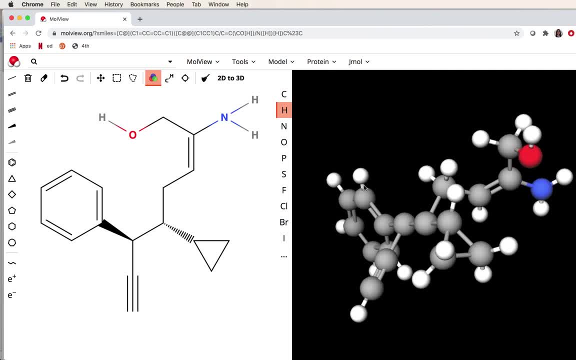 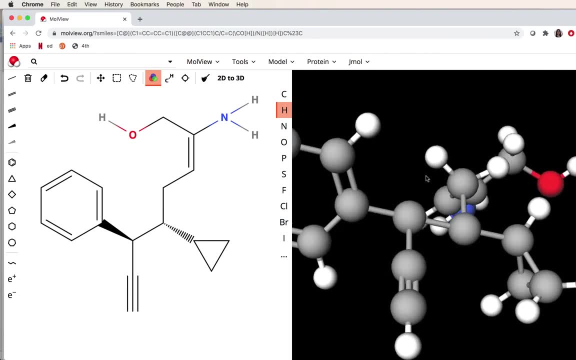 kind of representation. It may not be perfect, but it will at least be better than nothing, so that you can see a 3D model. Now, there is one flaw that I see, and this is a problem with MoldView and probably some of the other free drawing programs. The geometry on this carbon right here. 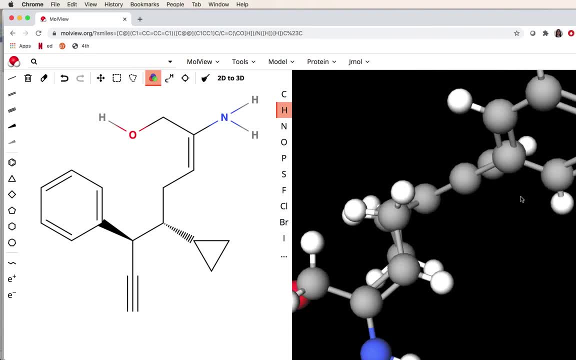 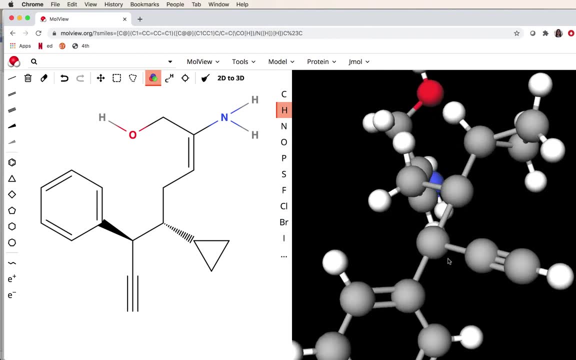 is not good. You can tell that because see how it's very flat. It's very flat there. If you built a model for that, you wouldn't have a flat geometry there. It would have to be much more tetrahedral. So there are going to be a few little things that aren't quite right with it, So just 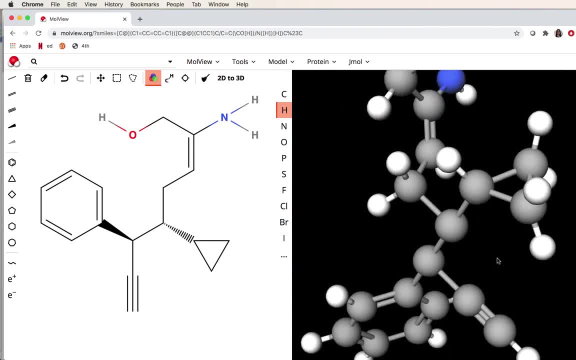 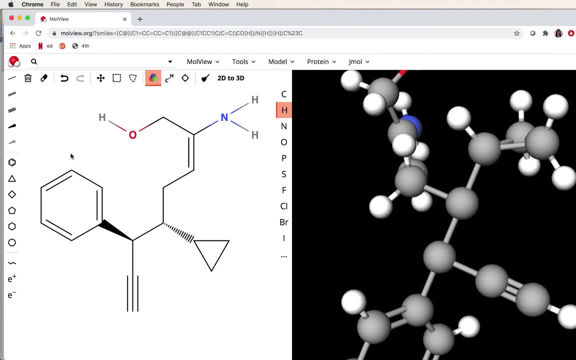 keep an eye out for that. But for you know, for a beginning user, it's really going to be fine. You'll get most of the way there And if you're building simple molecules, you usually won't have any problems. All right, So we're going to go ahead and start over again. I'm going to clear. 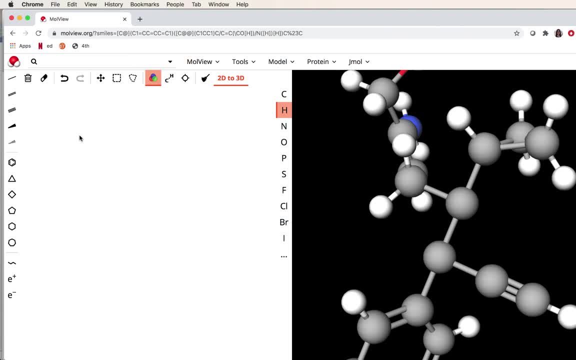 this and I'm going to go ahead and build an amino acid And I want to show the ability for charge here. So let's go ahead and we'll just build a glycine or something at first. So again, select the single bond. We're going to put a few atom, a few connections here. I'm going to go ahead and 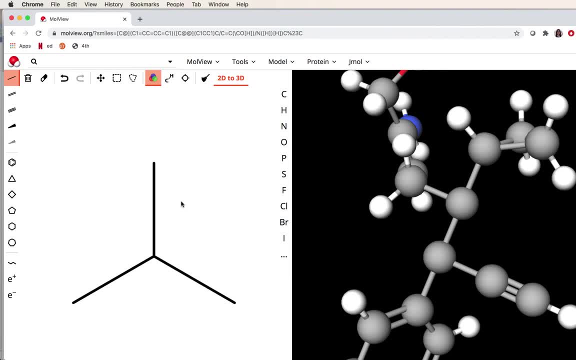 well, we'll build an alanine- maybe I'm going to click this to get us a little bit closer- And let's go ahead and fill out our different atoms that are part of our alanine. So our alanine has nitrogens in it. It has a nitrogen on the left side. It has a double bonded carbon over there. 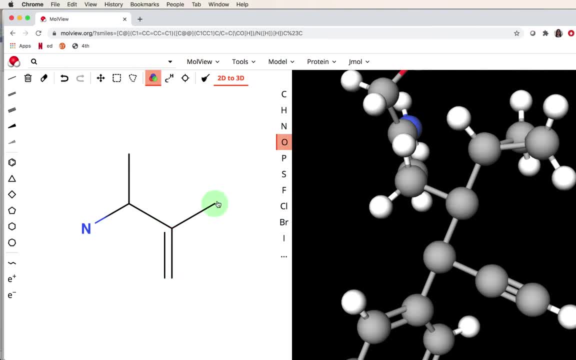 We need one more single bond And then let's fill in our oxygen. So this is the carboxylic acid over there, And that's it. We need some hydrogens on our nitrogen right Because of our 4-3-2-1. 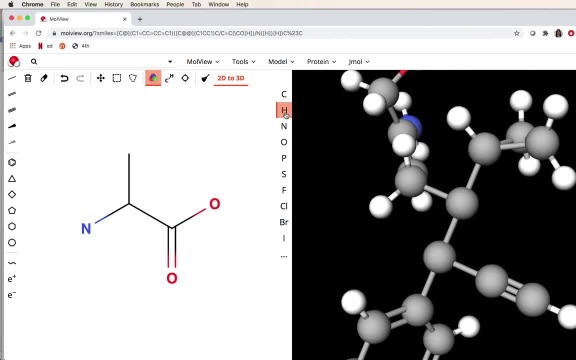 rule. we can't just have a single nitrogen like that. So I'm going to hit the hydrogen, hit the single bond and I'm going to put in three bonds because actually we're going to be drawing the positive charged version of nitrogen. And when you get to the amino acid chapter. 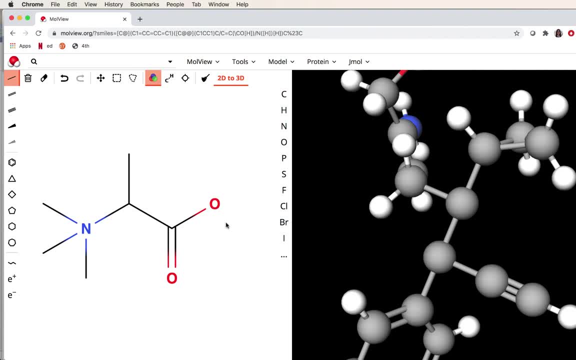 you'll learn all about that. We're also going to be dealing with the negatively charged oxygen, So this is a little bit more advanced than the very first two lessons. This is something we learn more about later: how we can have different numbers of bonds on certain elements because of 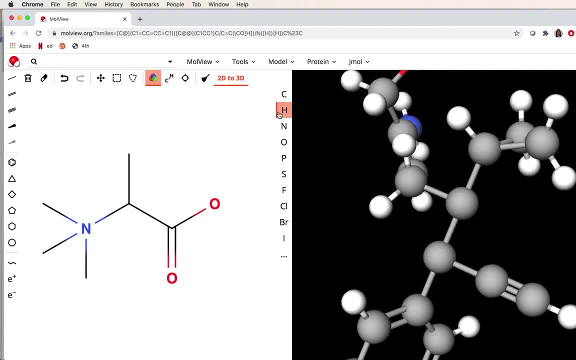 acid-based chemistry. So let's say we wanted to- oh, I forgot the hydrogens- Put our hydrogens on each H. Those are going to be carbons, unless you selected the hydrogen there. And oh, one other thing I wanted to show you. See this thing here: C to H, That's going to fill in all the hydrogens. 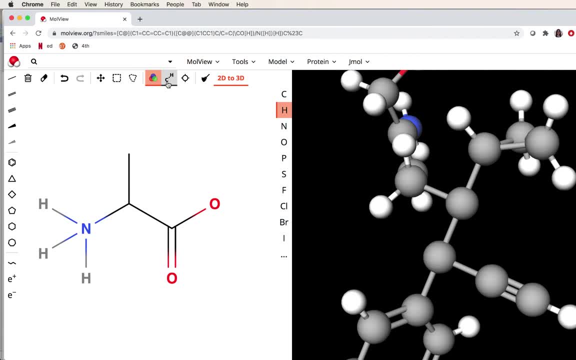 So we kind of make a big deal about it in, I think, unit five, where we look at the professional drawing style of organic chemistry, where we leave out a lot of stuff. It's like we kind of assume that you know that there's carbons and we assume that you know there's hydrogens here, But when 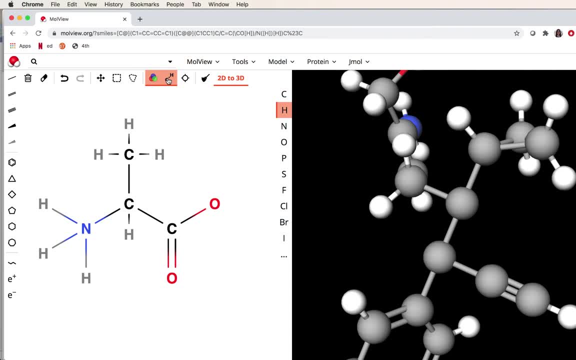 you click this button, it gives us the kind of simpler version of that. So we're going to put in the hydrogen version, kind of like I show you in those animations, shows you where all the carbons are, shows you where all the hydrogens are. So that can be useful for people in the 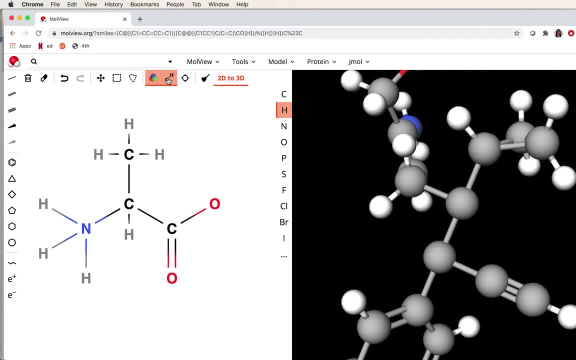 beginning to reveal what's really behind the professional drawing. Okay, so that's it. We need to show the charges. You maybe want to practice the charges. Let's put the positive charge there, the negative charge there. If you need to get rid of the charges, you're going to. 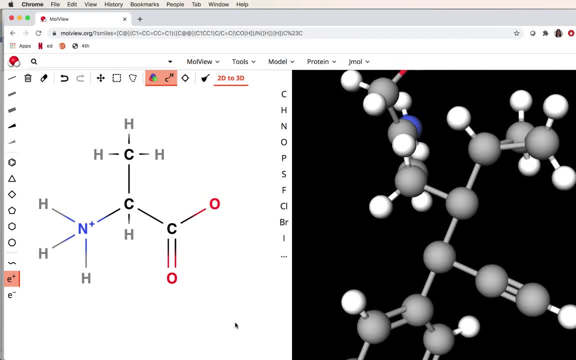 just do some addition. basically, Let's add the plus plus, It goes away. We don't really do this, but you could have a positive charge option. Okay, you could have a double charge. So the more you click this, the more charges change. But 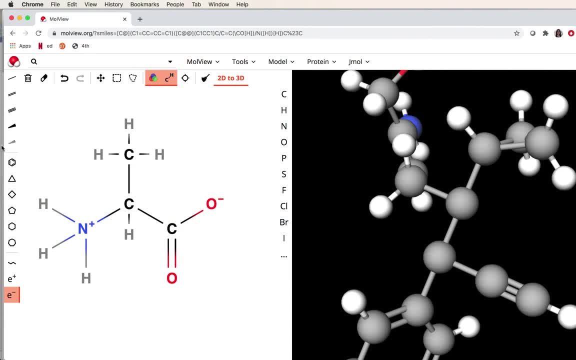 that's the one we need right there. If you want to draw this very good, very properly, you can put the stereochemistry in. So that's technically a nicely drawn alanine. You may want to capture that image. if you want to keep track of these or draw them, You could probably do a screenshot. 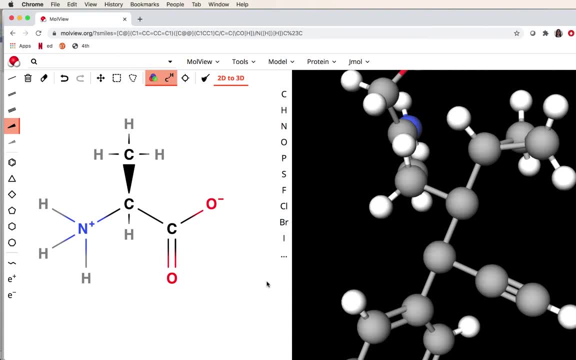 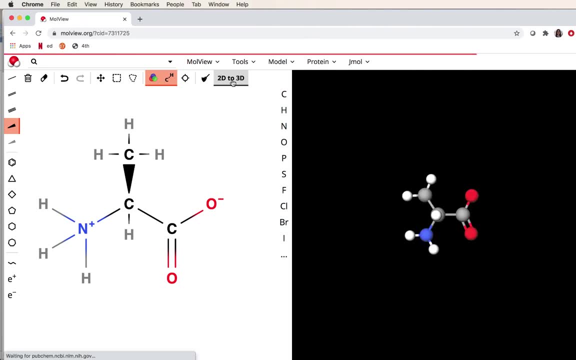 and capture that alanine so that you can maybe collect all your amino acids. Let's go ahead and see what happens when we do the 2D to 3D. So this might be what you would do if you don't have a model kit to build with our alanines. All right, so let's see what MOLVU did for us. 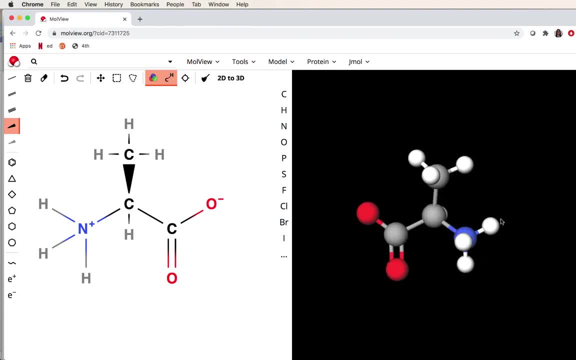 Okay, just like I said before, it's better than nothing, but it does do a little bit of things that aren't super quite right. The one problem that it does is it doesn't seem to know about the stereochemistry very well. It's actually given us the reverse stereochem, So instead of the 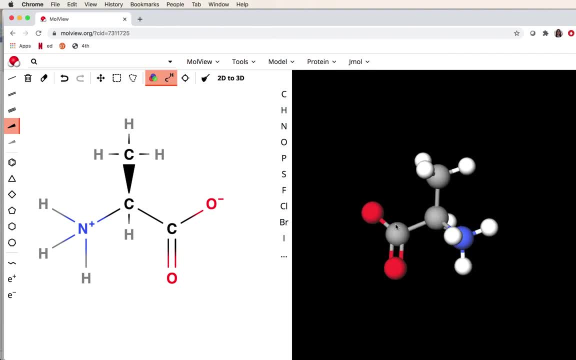 L-amino acid. this has given us the R-amino acid, So unfortunately I don't know how to fix this. If someone can figure out how to get it to do the correct, the stereochemistry, please let me know and we'll make a note of it. But you know, like I said, 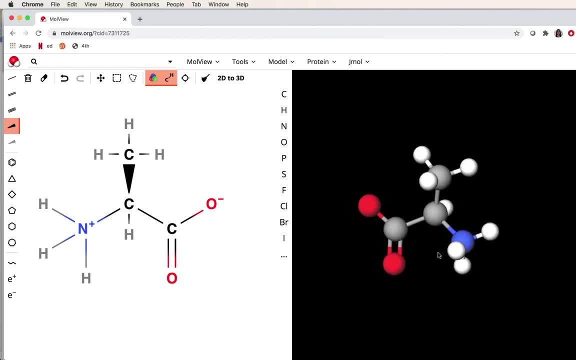 it's better than nothing. So for a beginning student, at least you have a model, I mean. that's why I said it's always better to have a model kit. but some people just can't have a model kit, Some people can't have Pymol, So this is at least better than not having anything. 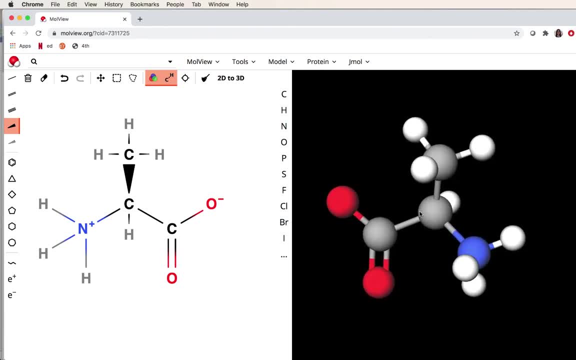 So the only problem with this is we have the wrong stereochemistry here, But other than that it's really fine. We have the three hydrogens on our nitrogen. Everything else looks just fine. Let's go ahead and build this out a little bit more, just for fun. 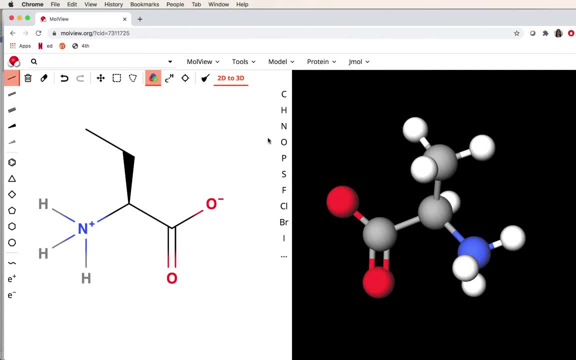 Let's turn this into maybe a threonine or something. So we're going to do oxygen. This is going to be the threonine. Put another hydrogen here, OK, so now we've turned our alanine into a threonine, right? The stereochem is this, I believe. 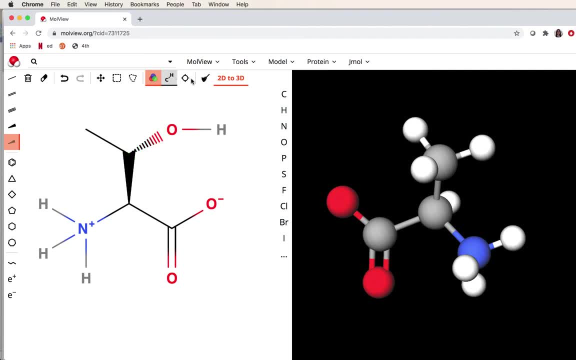 That's the correct stereochem. And then let's do the look at where the hydrogens are. OK, that's cool, Just see that. And let's do the threonine and see what it does. And now we have made a threonine for ourselves, Let's orient it correctly. 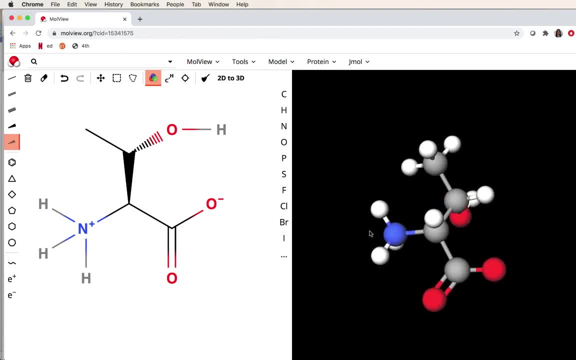 And again it's giving me the, the wrong stereochem, the wrong isomer. I don't know why, but it's still OK. It's a threonine. OK, it's the wrong threonine, but that's all right. 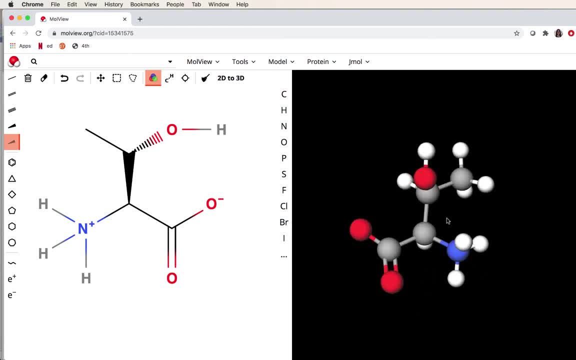 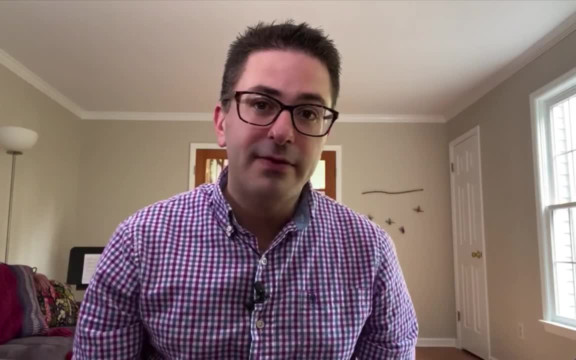 So that's how you build amino acids. Again, two fingers zooms in and out on this picture. Same thing here. We can make this bigger, smaller. So those are some of the important drawing features of MOLView. There is also an amazing feature that PyMOL doesn't have that we're going to check out right now. 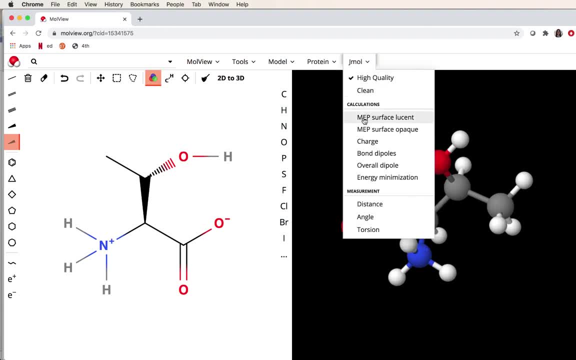 If you go to this JMOL menu, you're going to be able to see some really cool things that to do This MEP is particularly interesting. This is the molecular electrostatic potential surface, And now what that means. electrostatic potential is having to do with the charge that shows up on the surface in the different areas of the molecule. 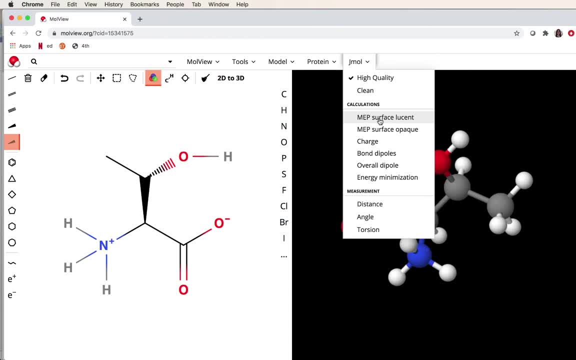 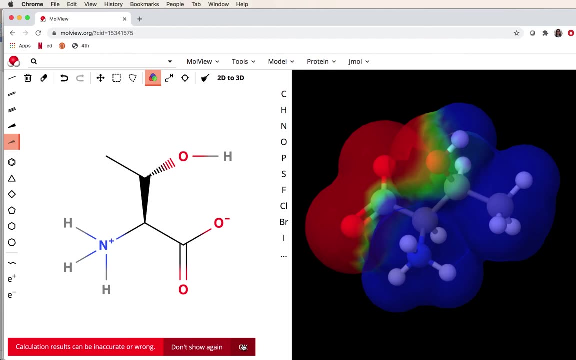 So areas that are very negatively charged, that are rich in a lone pair electrons, for example, those are going to have a red color. Areas that don't have a lot of charge to them, that are maybe nonpolar or positive charge, are going to be a blue color. So I'm going to show you what will show up here when we get that. 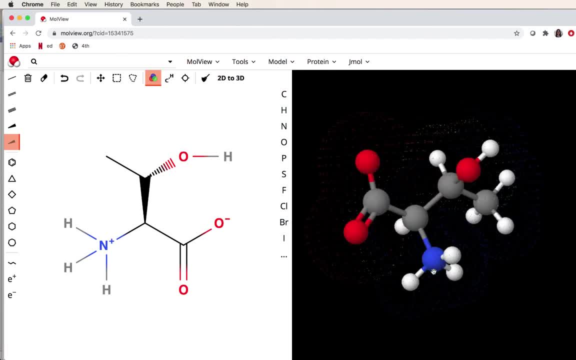 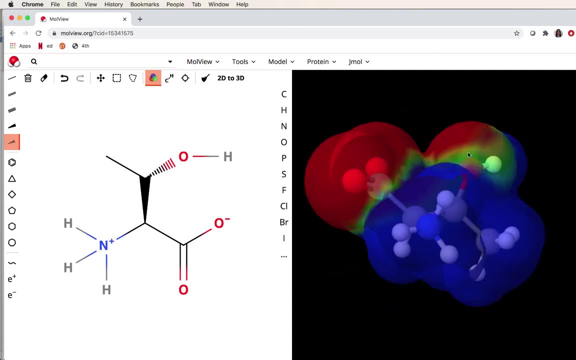 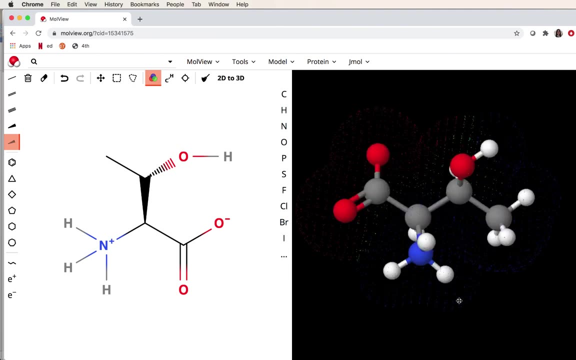 Now this is super cool to see this. This is actually very, very useful for chemists to look at the properties of a molecule. So what we see here: the carboxylate and then the alcohol parts are rendered in red. So we can see there's a lot of electron density, a lot of lone pair electrons over there. 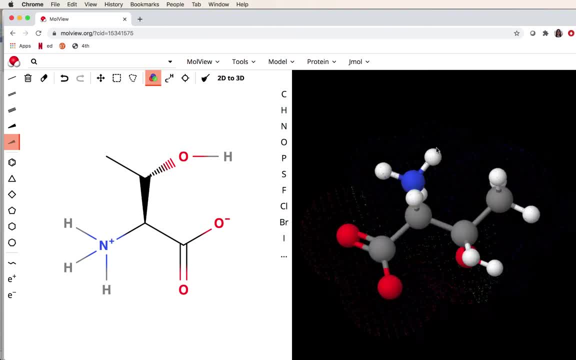 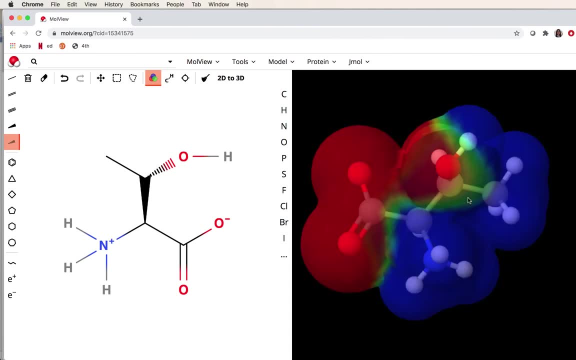 And then the blue parts, which is where the ammonium and then this methyl group are. these are blue because there's actually not a lot of electron density there. So you know, you can probably see this without this electropotential surface. 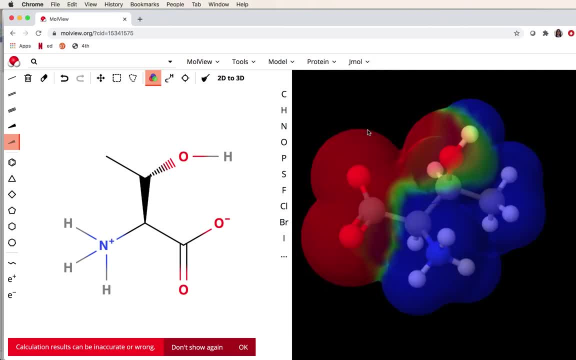 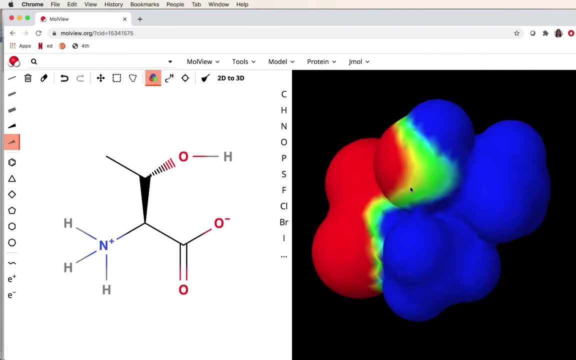 but it's still kind of really cool to see that There's two different versions of it. There's an opaque version and a translucent version, So this is very cool. A lot of organic chemistry books will show you things like this, So this is really cool. 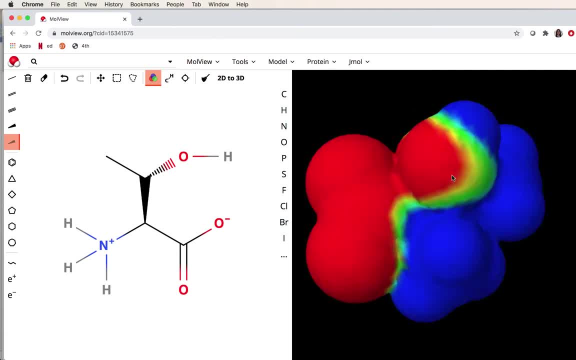 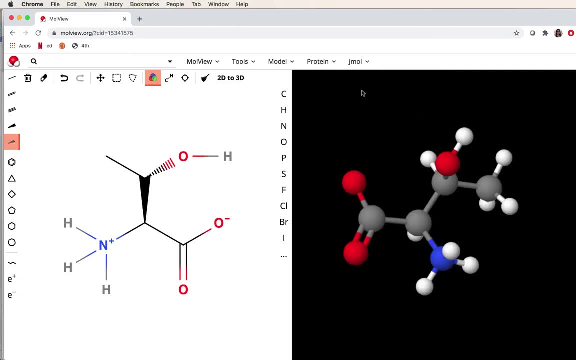 This can help you. give you give clues about where hydrogen bonding will occur. Hydrogen bonding will occur between blue and red regions, basically between different molecules, So that's really cool. If you want to turn that off, you go ahead and hit clean. 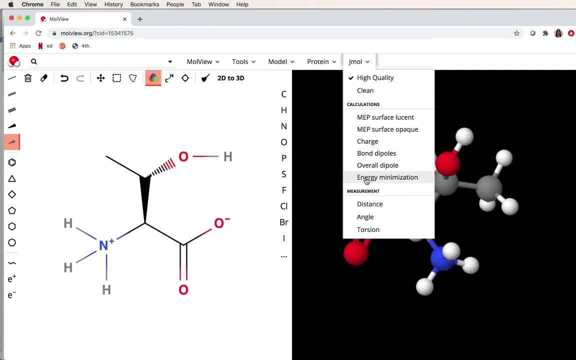 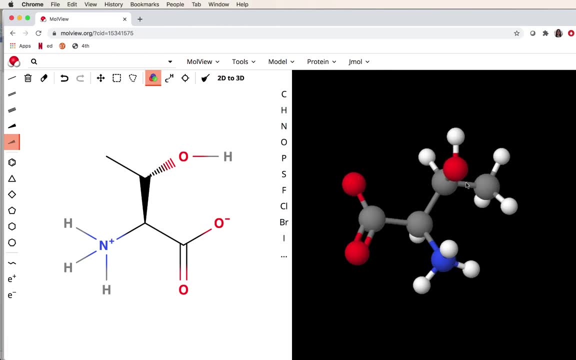 There's other things we can look at. We can look at the overall dipole, energy minimization, which may help to minimize any kind of strain that's in your molecules. So see how it's kind of shaking and shuddering a little bit. 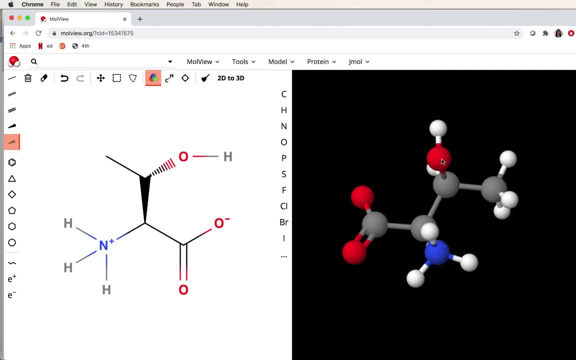 That's because it's doing some energy minimization, And we do have another video using Pymol. that's all about energy minimization, where we build that creative amino acid. We do that at the end, So that's something to know about also. 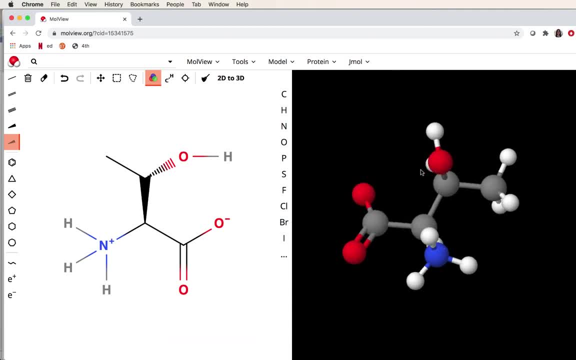 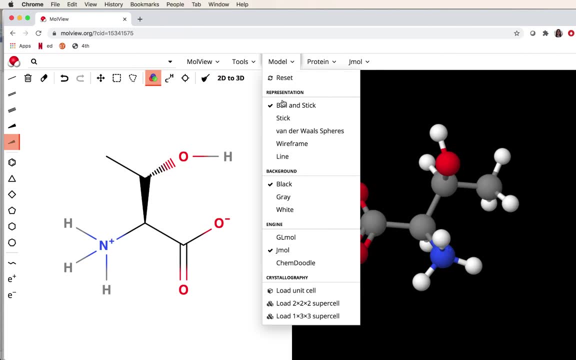 If your structure kind of looks a little bit crazy, maybe you need to do some energy minimization. So I'm going to probably turn this off. I'm going to turn that off there. Other things that we can do. we can change what the model looks like. 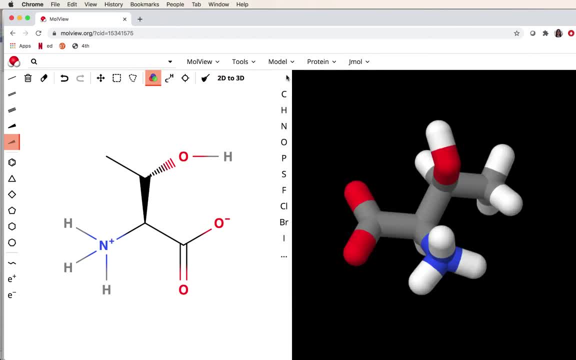 We can change it from ball and stick to just like these kind of bigger sticks. We can look at the. there's this little thing here. It's the cleanup feature. This is going to kind of make the molecule look a little bit better. 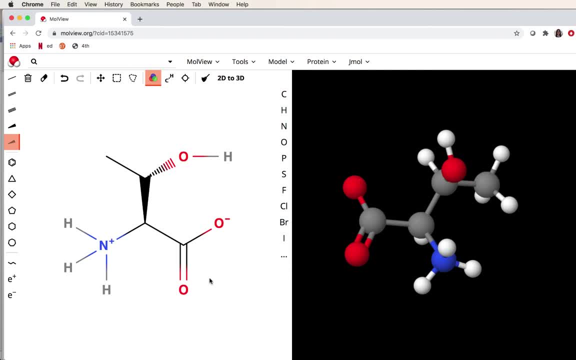 If you've done a lot of overlapping bonds or you've kind of gone a little crazy with how you draw your bonds, you may need to use this feature. It's kind of like a spell check and it kind of reorients it. 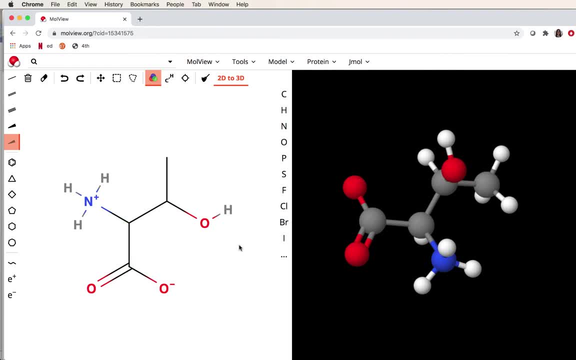 I didn't need to do it here, And actually here it makes it worse honestly, But you may want to use that if your structure gets a little bit wild. That's the cleanup feature, All right, so anyway, by the way, also erasing. 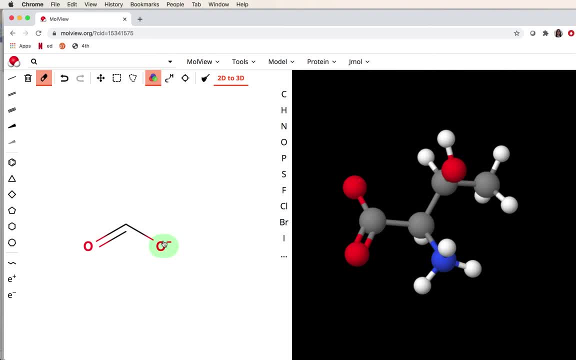 You can also erase things, OK. so it's kind of intuitive, It's kind of like a paint sort of program, but for molecules. So what I want to do now- so we're going to erase everything- I want to show you the really powerful part of MOL-View, which is great. 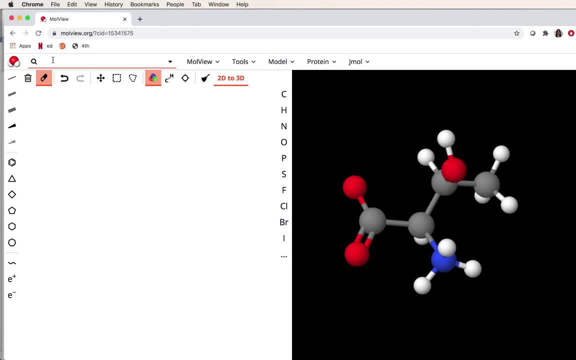 especially if you don't have models. And even if you do have models, you can look at anything you want. It's really amazing. We can search for things And PyMOL doesn't do this. You can do it manually in PyMOL, but this program. 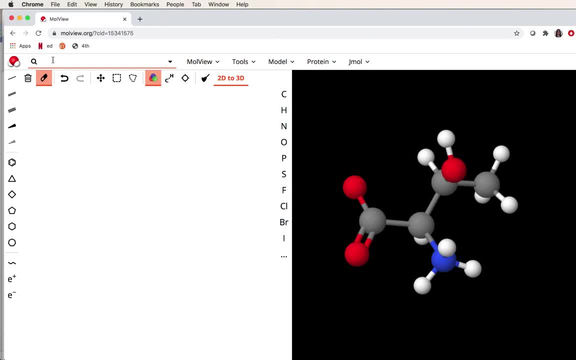 uses the cloud to store I don't know how many structures, enormous amount of structures. Let's say you're just doing chapter one and you want to look at methane. You don't have a model kit or PyMOL, but you want to look at methane. 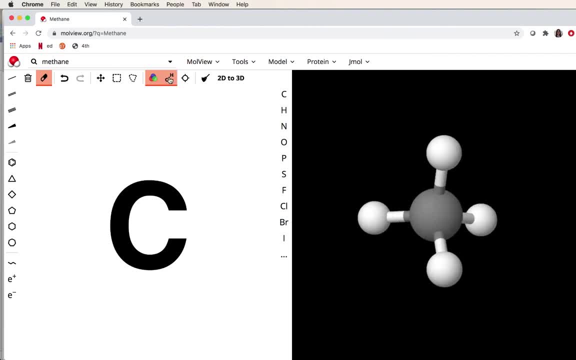 Methane will just show up here for you. So there's our methane, We can show the hydrogens, And so we have a drawing of methane and we have our 3D molecule of methane. OK, what else can we do? 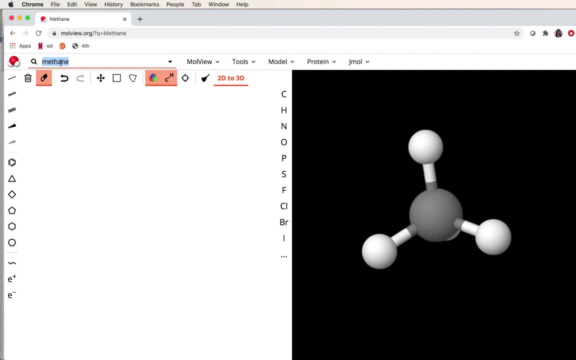 Let's look up Some more complicated molecules. Let's look up chlorophyll. Let's see what comes up with chlorophyll. OK, let's do chlorophyll A. We get a giant structure, your very own chlorophyll. 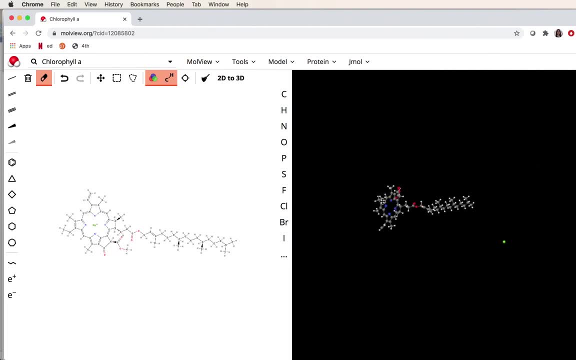 Look at that. So that's something that most students would not really be able to build because we would need a lot of model kits for that. But that is chlorophyll. It's got a very heme-like top to it And it has a very hydrophobic, carbon-rich tail. 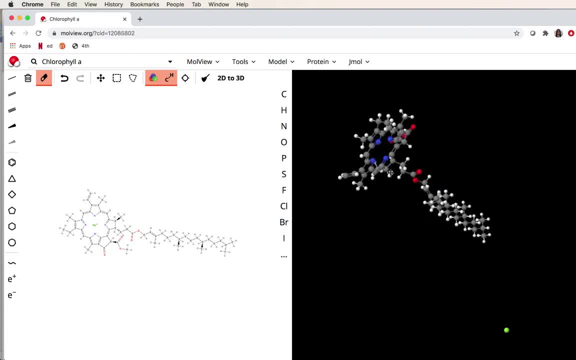 It's also called an isoprene tail. So there's our structure of chlorophyll And you can kind of zoom up to it and figure out how to move it around, The one kind of little error that it makes again, see this little thing here. 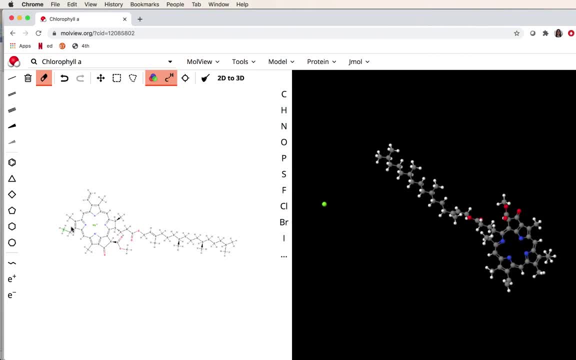 That's supposed to be a magnesium and that's supposed to be in the ring here. We can see it better over here. See how there's actually supposed to be a magnesium inside the chlorine ring. Oops, I just erased it. There's a little magnesium. 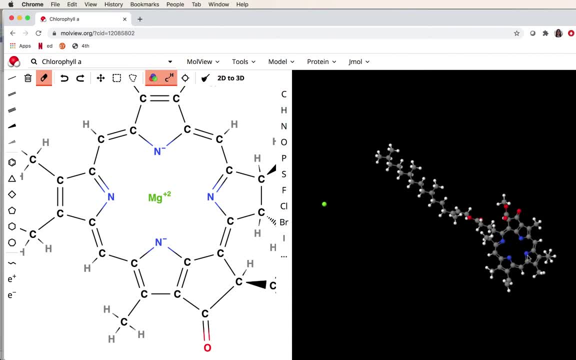 So I don't know why, but the magnesium is not where it's supposed to be. So, like I said, it's a free program. You get what you get with it, But there may be some way to fix that. I'm really not sure. 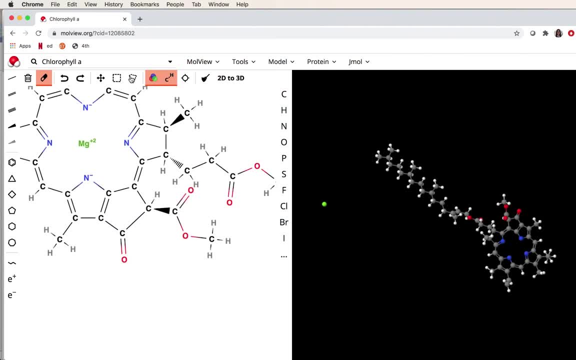 But I've noticed that kind of a problem with it. But this is really cool. If you want to, just you can. maybe obviously you can change this- put a phosphorus here or something silly like that, So you can use this as a beginning for drawing things. 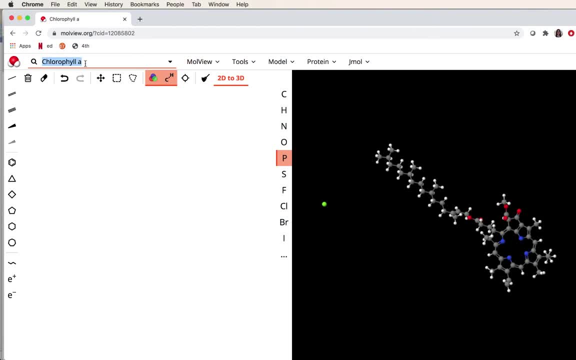 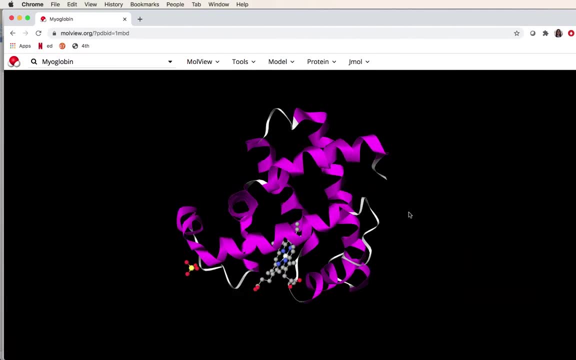 Let's see what else we can do. We can look at maybe a protein. even Let's try out myoglobin. Myoglobin- Everything's in here. It's amazing: There's our myoglobin. So this is one of the molecules that we are studying. 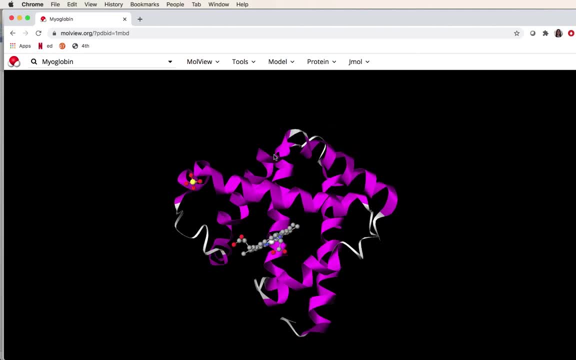 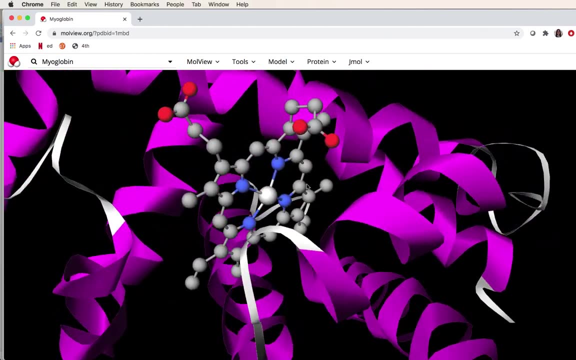 We're studying hemoglobin a lot in the course. Hemoglobin keeps coming back in many of the lessons, So myoglobin is a smaller version of hemoglobin And we can see our heme. So, yeah, so first lesson if you don't have PyMOL. 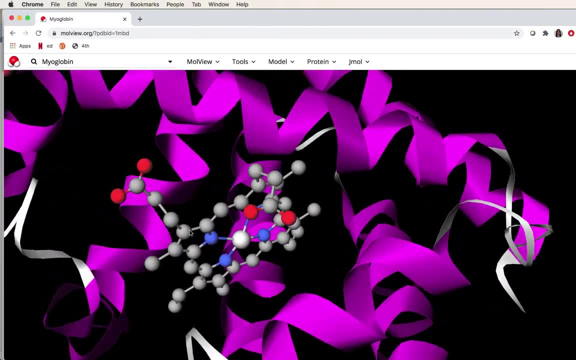 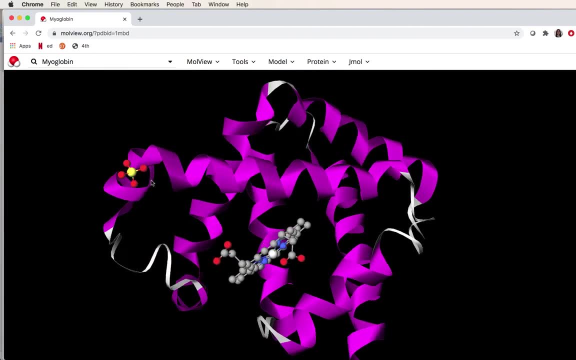 if you don't have the model kit, we can still get something out of looking at 3D molecules And we can see the heme in there And we can see the alpha helix. There's a little sulfate group here which actually 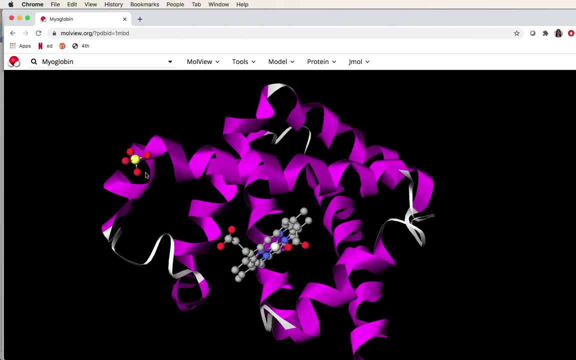 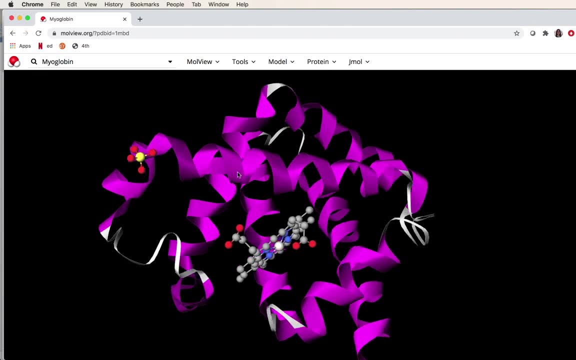 doesn't do anything. The reason it's there is because the crystal structure that the MOL-View is drawing on has this just random molecule sitting there. It doesn't do anything biologically, But it's just kind of taking information that it's getting from the crystal structure database. 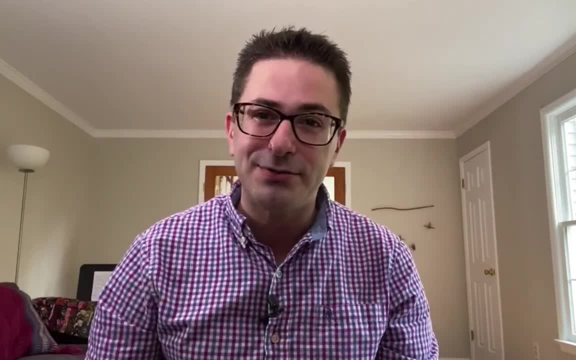 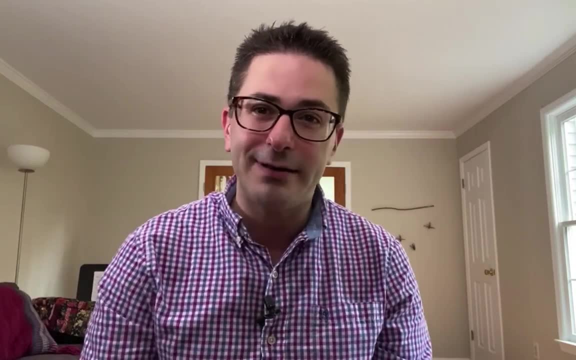 OK, I hope that you found that tutorial interesting and that it inspired you to begin using MOL-View to draw and render molecules in 3D. even if you have a model kit or PyMOL, It's a great resource to have, especially since you. 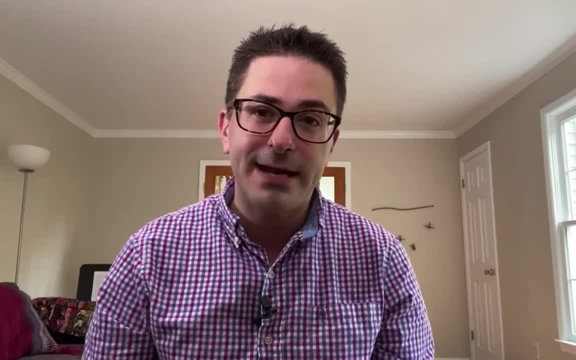 can draw on this cloud-based database to load all kinds of structures and easily view them. Thank you. 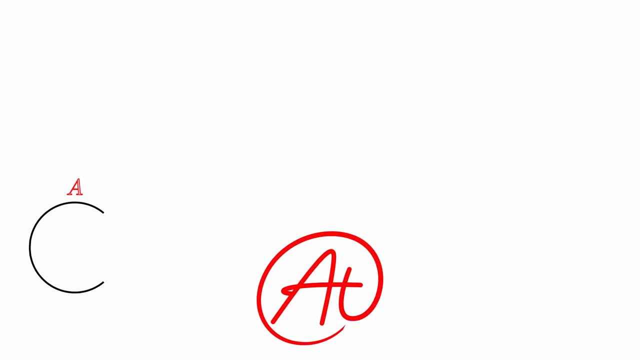 Hey guys, it's Mark from Ace Tutors, and in this video I'm going to quickly explain a concept that many students, including myself, have struggled with, And that's the difference between events being mutually exclusive versus independent. So first let's start with events being mutually.